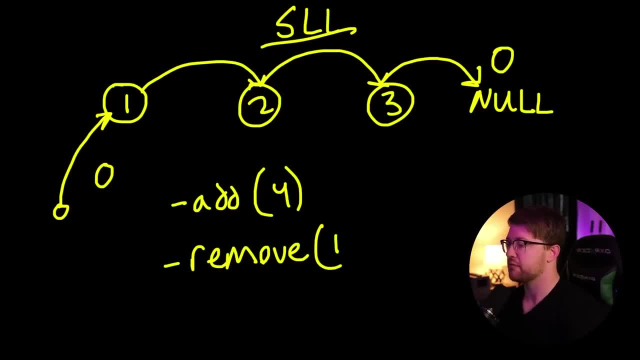 called remove. that removes an element that matches some values. If we wanted to remove one, we could write the operation that removes this list And then, finally, we have insert. So we can say that we want to insert value three at position two, and there's an operation we can do as well to make. 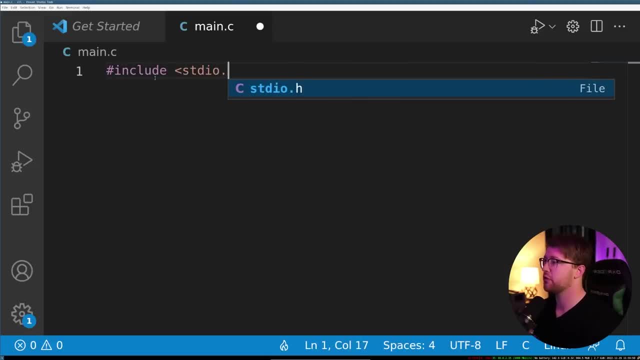 that happen Here in our code editor. we're going to get started on our code. So we start with the boilerplate C stuff int main, arg C, arg V and return zero. So the first thing we have to do is: 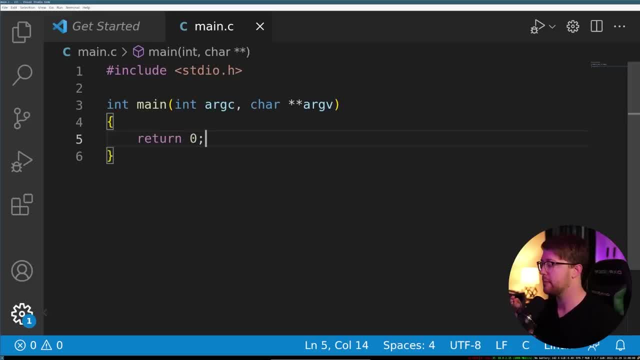 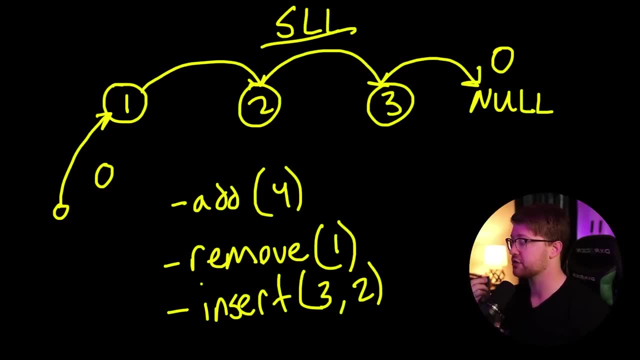 create the structure that represents a single node in our list. Remember before, like we saw in our drawing, a linked list is just a series of nodes that are connected to each other. So we have to go through and actually define that node structure. in C We're going to type the following code: 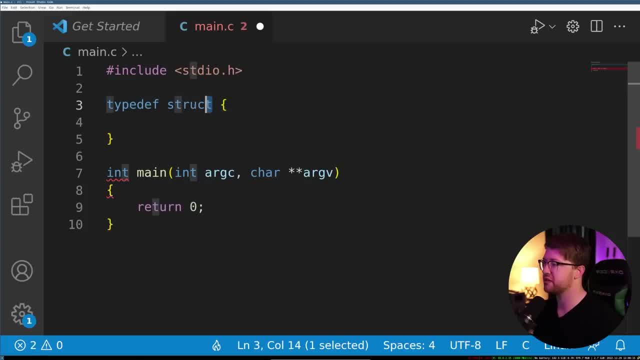 typedef struct. And the reason we do a typedef struct is it removes the necessity to type struct before every use of the structure. right, If we didn't say that we wouldn't be able to typedef struct, We would have to type struct in the front, And I find that kind of annoying. So 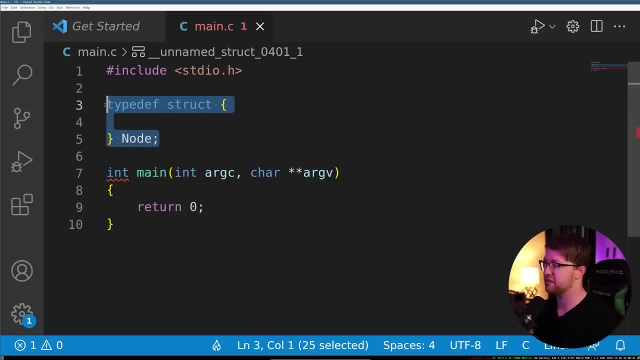 typedef struct node, and that is going to represent a single node in our list. Inside of that node, we have two things: We have a void pointer, which points to the next element in the list, And then we also have int data, So this will contain the data that we're tracking in our list. 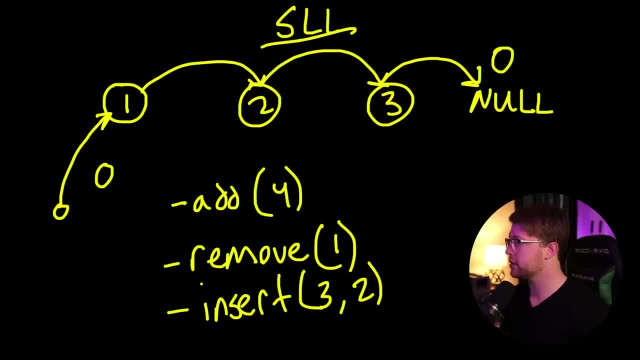 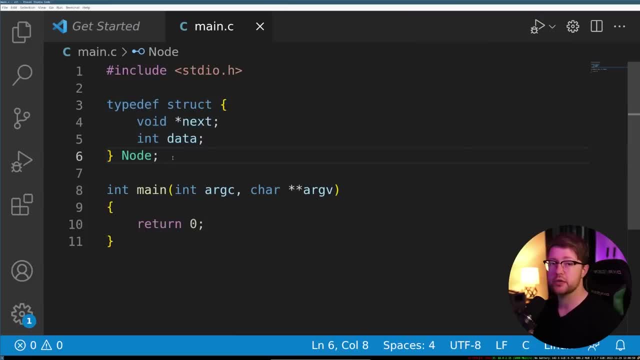 Again, looking at our drawing here we have node one. Node one will be the data, And then that next element is going to be the data, And that's all we need in terms of new structures to make our list happen. Also, we need a node pointer, that is, the head of the list. that represents the first. 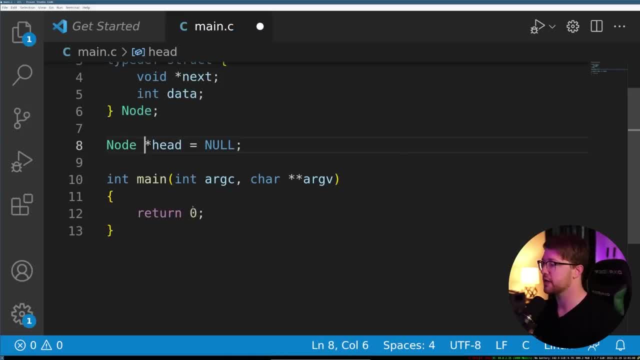 point that points into our list And that will be null to begin. So now that we have all of those structures set up, we can actually write the code that does our operations, And again those operations are going to be a function to add a node to the list, to remove a node from the list. 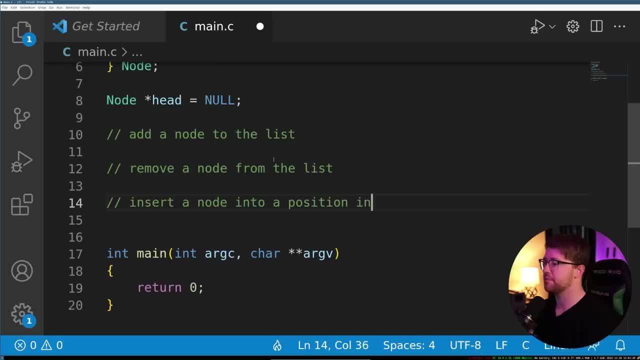 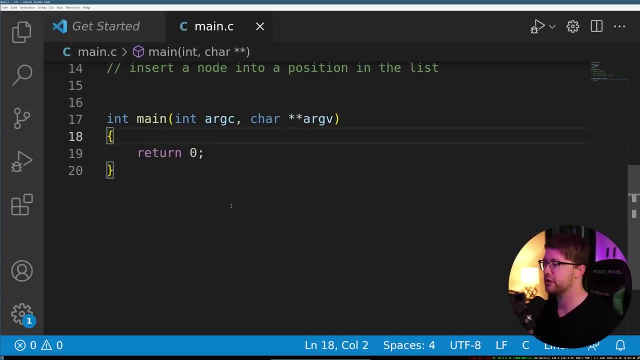 to insert a node into a position in the list. So what we'll do is we'll write those functions, but we need to do that first. So we're going to do that first. So we're going to do that first. So we need to actually create a way for the user to interact with the list, So we are going to prompt. 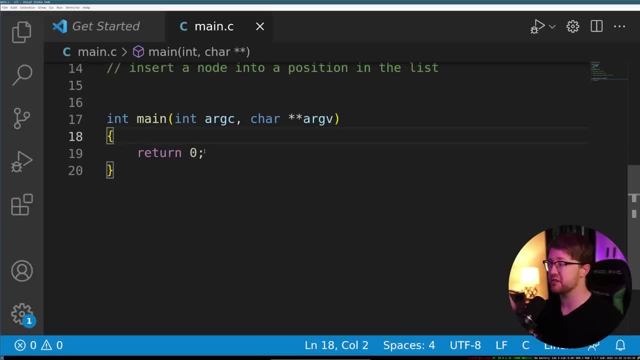 the user for a number of options to either add, remove or insert from the list. But first we have to give them a menu. So we'll say print menu And that menu function is just going to literally print all the ops. So we'll say void, print menu And the option is going to be: you have the 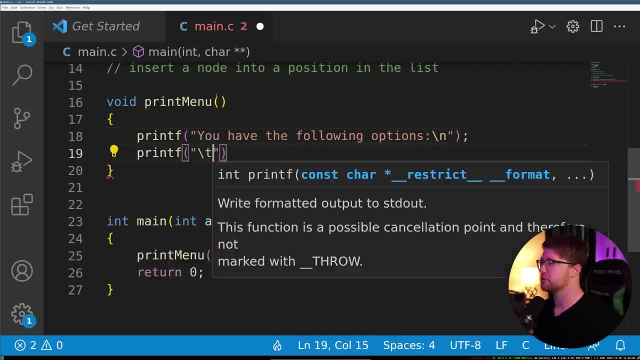 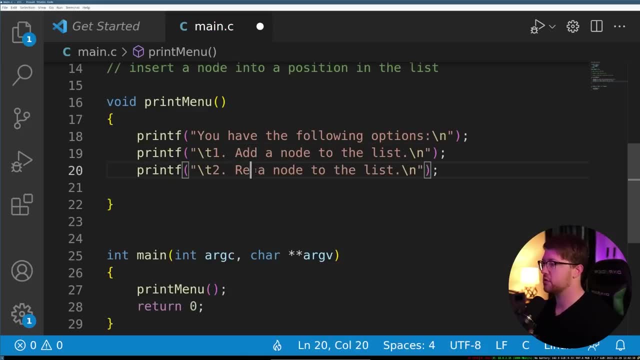 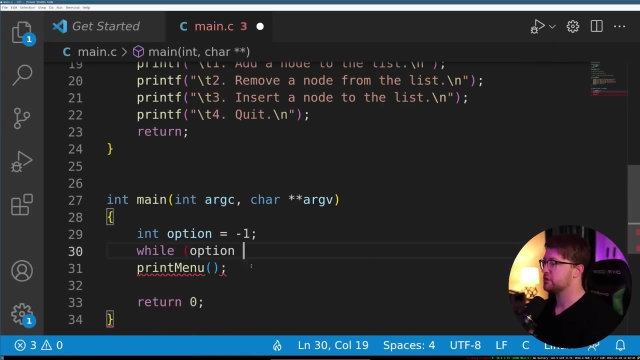 following options: To add a node to the list to is to remove a node from the list. So we're going to say to remove a node from the list. Third is to insert a node to the list And then the fourth is to just quit And then we'll return our int option is, while option is not equal to for we will print. 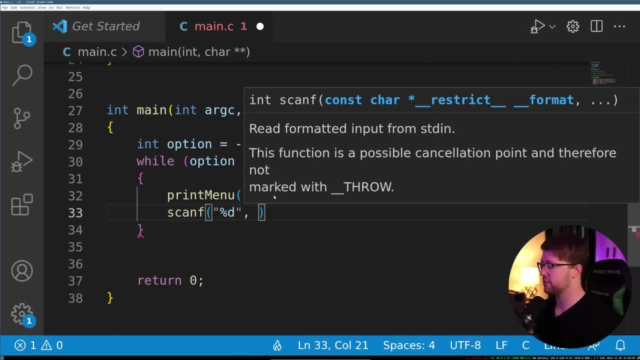 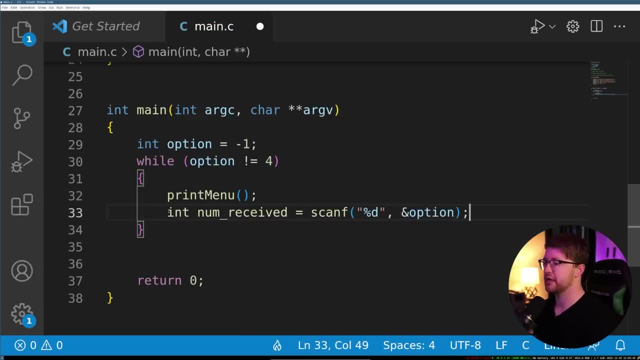 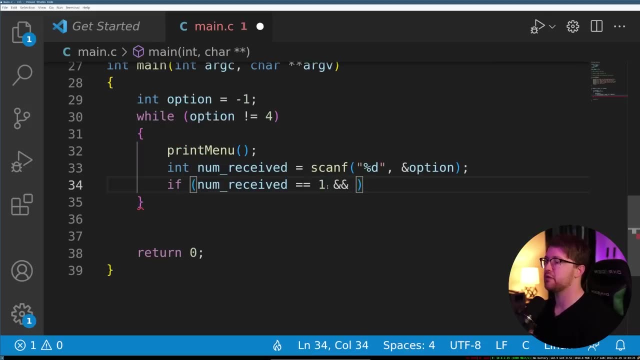 the menu. We will scan F, store that in our option variable And we'll say that int num received equals scan F and if numReceived is equal to one, which means that we got a value back from the user, and also if the option is greater than zero. 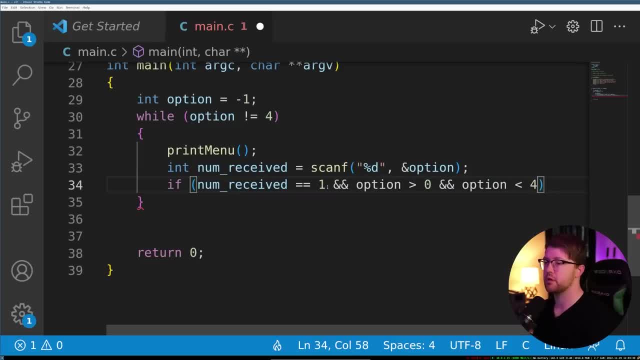 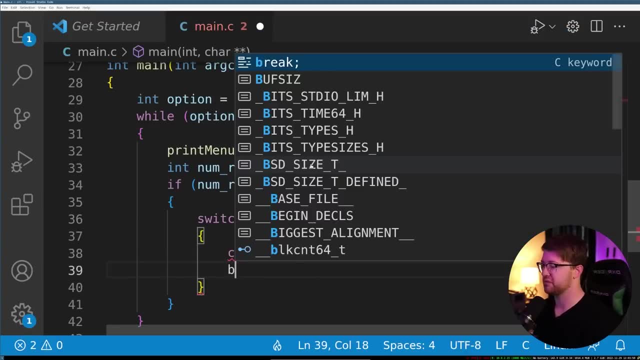 and if the option is less than four, So we'll make a switch statement that switches the following things. we're allowed to do So switch option: in the case that it is four, we'll just break. In the case that it's one, we will do our add operation. 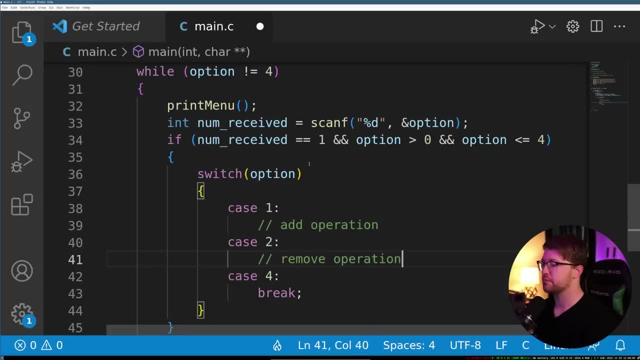 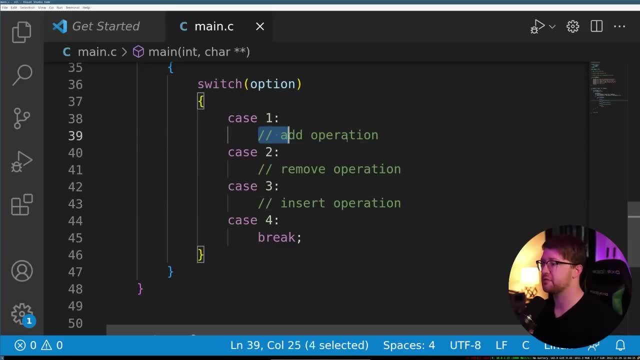 Function. case two: remove operation. case three: insert operation. and that's it So pretty straightforward. Now we have to actually write these functions, The function that we're gonna use to add a node to the list we're gonna define here. 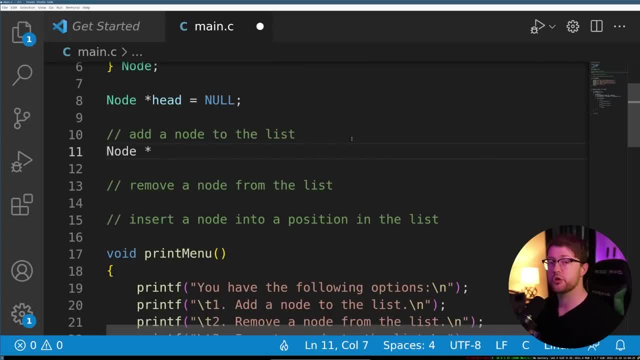 And we're going to have that function return a pointer to the node that it returns, We're gonna say node pointer, add node And we're gonna say that the add node function takes an int data that we wanna add to that list. Okay, 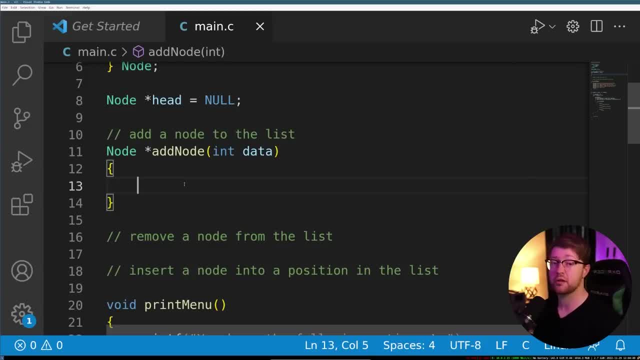 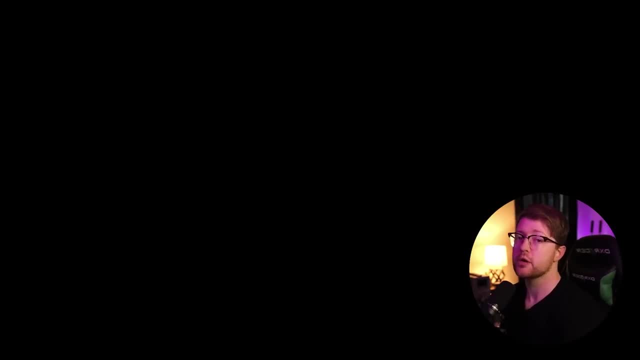 So the algorithm for adding a node to a linked list, it depends on a few edge cases. So we're gonna go back into Photoshop here and kind of talk about what those edge cases are. So you have two cases you have to worry about when you're adding a node to a list. 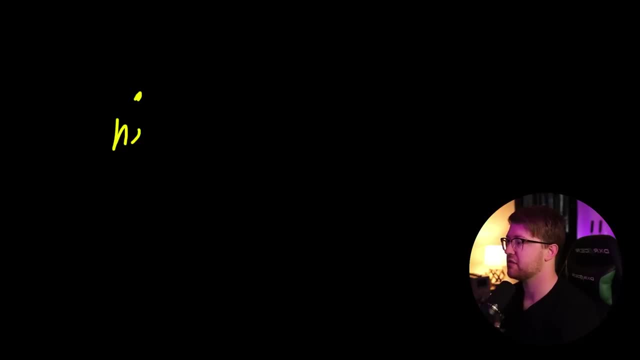 In the case that you have your head. remember the head is just the pointer to the rest of the list. If your head is equal to null, that means that you have an empty list. So all you have to do is allocate a node and then point the head to that node. 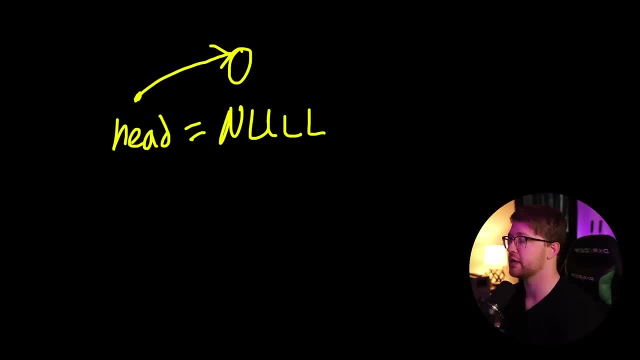 And that's it. That is the first insertion you get to do when you're adding a node to a linked list And then after that, if you have your head, that points out to a node that already exists and you wanna add an additional node. 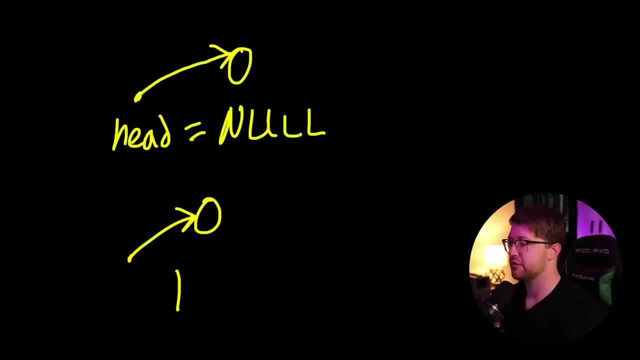 you could do this two ways. You can do what's called a insertion at the front or an addition at the front, which is a little more complicated, And the second is to add the node at the end. The problem with adding a node to the end of a list. 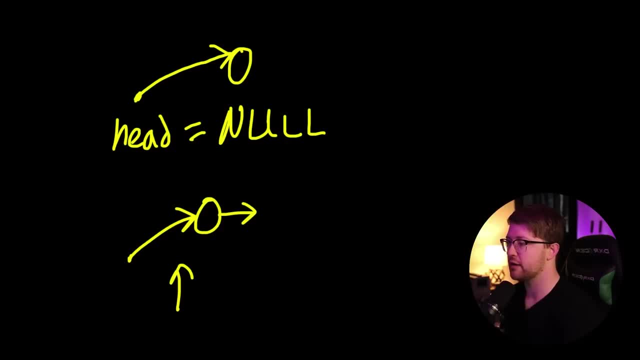 is that you have to walk the entire list to figure out where the final pointer is equal to null. This actually makes our algorithm end up being O of N, where every time we add a node to the list, we have to walk the entire length of the list. 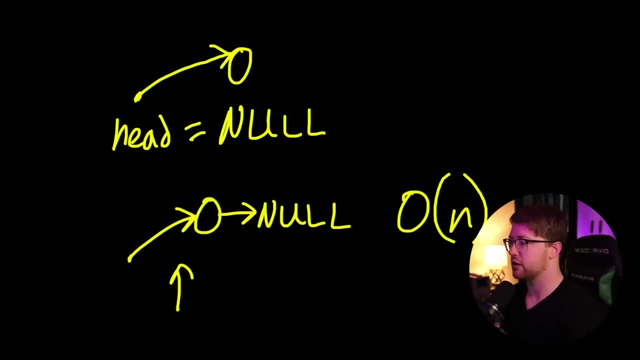 which could be incredibly long And over time that will bog down our computer. So the algorithm for doing a addition here is as follows. So we're gonna say again: this is our head and it's a little dot and it points out to our node here. 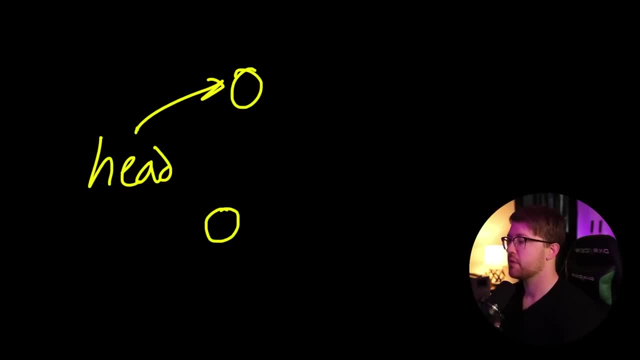 What we do is we first allocate a new node, We point the next pointer into the node to head, make them point to the same thing, And then we make head no longer point here And we say that head is equal to new node. 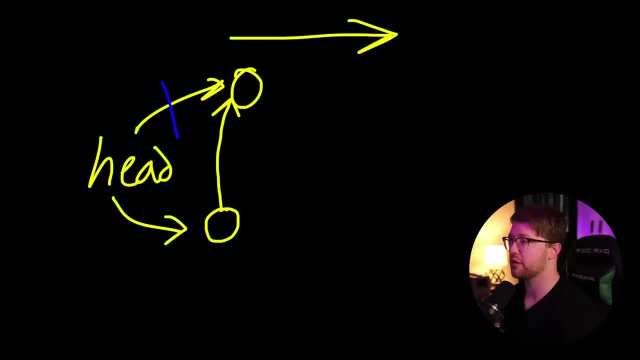 Effectively. this pushes the entire list forward this way and makes head point to our new node. So every time you do this, it doesn't depend on how long the list is, It always inserts it in O of one time, constant time operation. 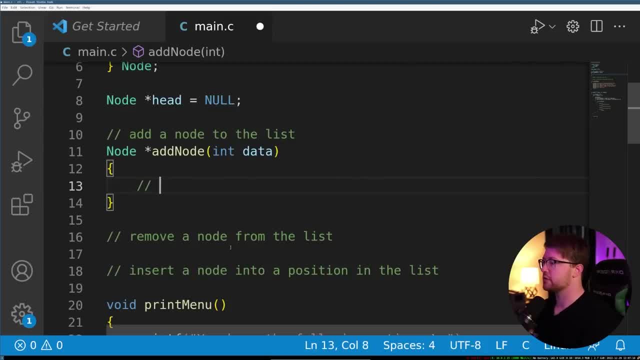 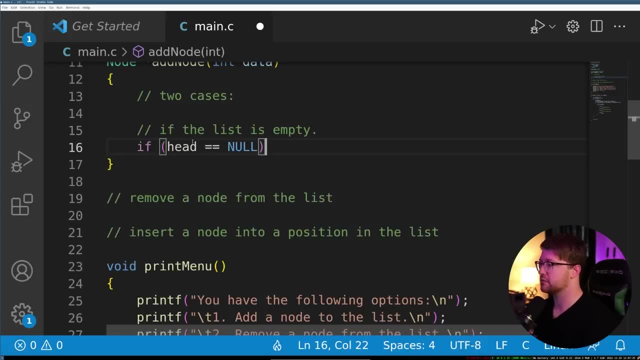 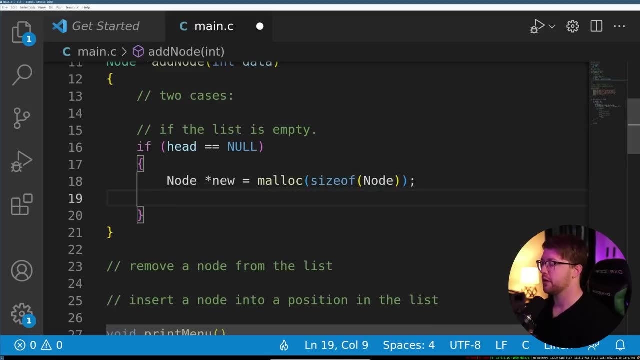 So let's make that algorithm happen right now. So again we have to handle our two cases. First is if the list is empty, If head double equals null node pointer new is equal to malloc size of node, And then always check to make sure. 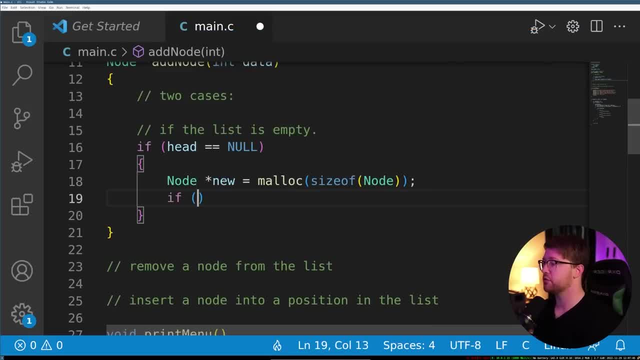 your pointers come back correct. So if new double equals null, it means that we had a significant issue in our malloc operation. We have to handle that, but not gonna worry too much about that. So we get back our pointer to our new node. 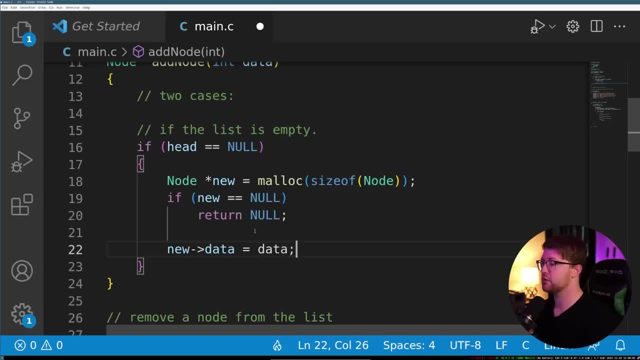 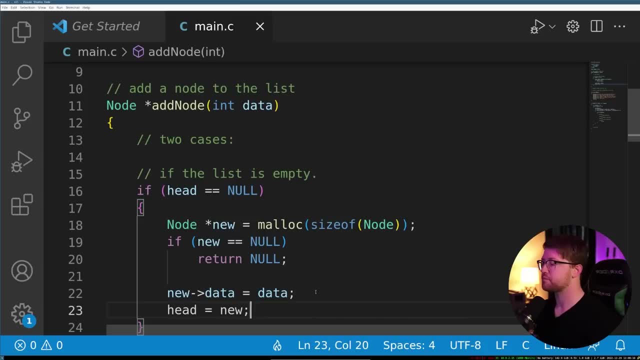 And we say that the new data is equal to data, which is the data from the user, that the value we're actually inserting into our list. and then we say that head equals new, so this will append the new node to the front of our list. and then, finally, we want to make sure that we set the new 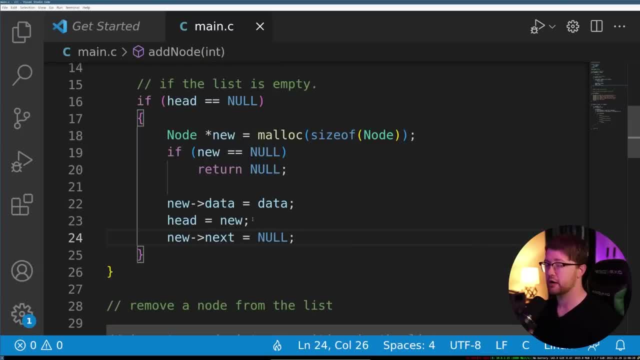 next equal to null, so this will take care of the list. if the list is empty, we're adding a singly, a single item to it, pretty straightforward. so otherwise, if the head is not null, it's a list that is not empty, we have to do our previous operation. so this is the same thing. we take this. 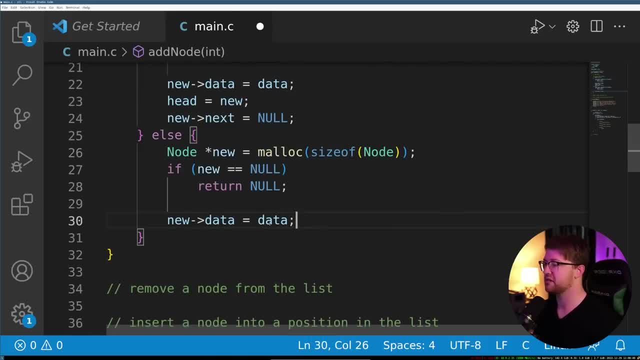 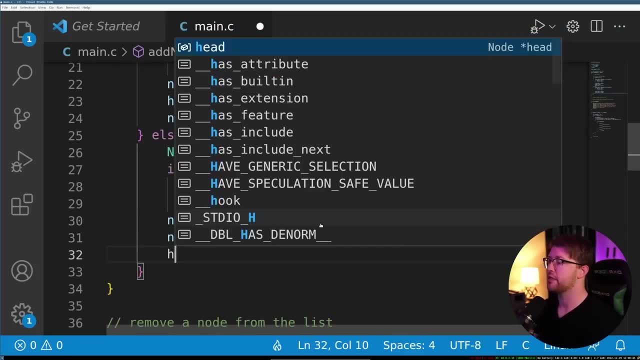 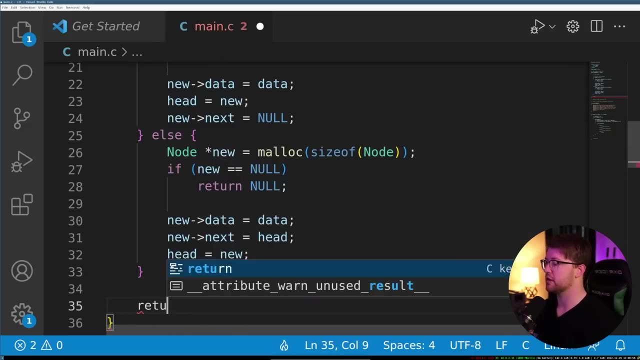 the malloc, a new node, and we say that the new data is equal to the data. then what we do is we say that the new next pointer is equal to the current head pointer, and then the head pointer is equal to new, and that's it. and then after that we return the new pointer. but to make this 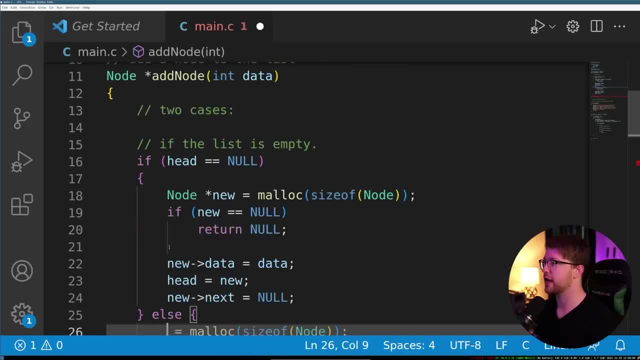 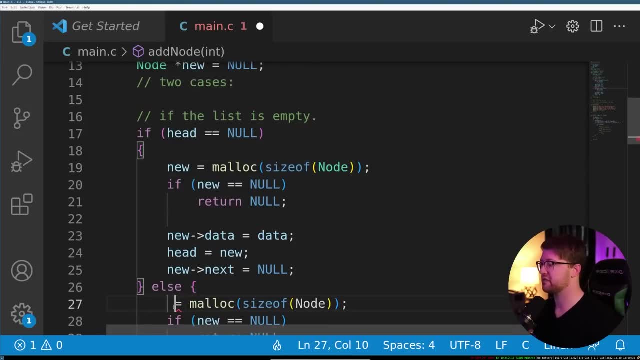 the correct scope. we actually have to move this node, new pointer out of this conditional statement, set it to null and then just say that new equals these mallocs. okay, that we have that. and then we return new. so now the user gets access to the new node if they. 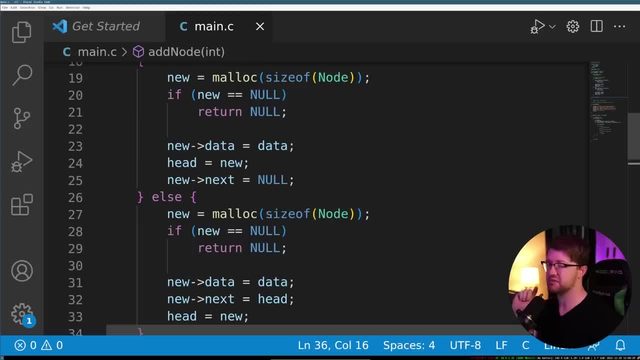 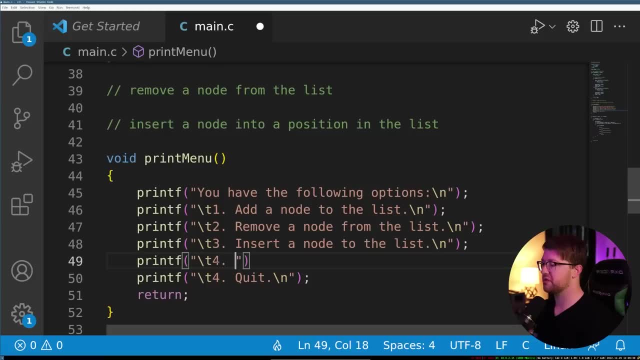 want to use it here. we've created the way to add a node to the list and we can add as many nodes as we want. we probably should create a way for the user to print the list right, so we'll add another option four. we'll say: print your list. we'll make five the quit and we'll change it so that if 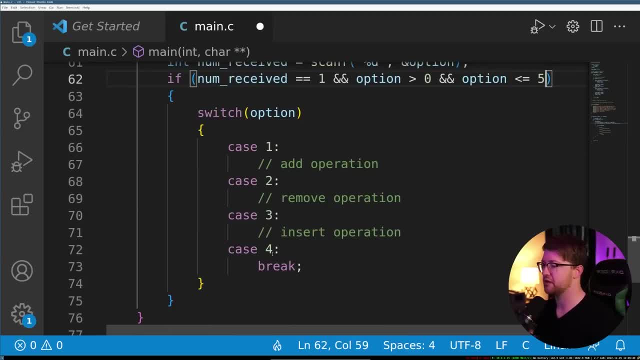 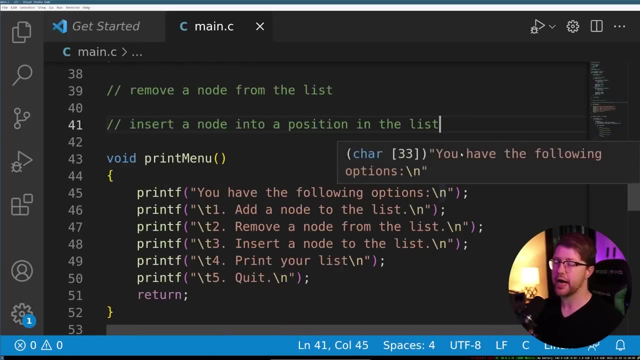 option is not equal to five and if it's greater than equal to five and then in case five we break and we'll say case four is our print the list. so we've created the operation to add an element to the list very easy so we can test this real quick. so i want to test out our add operation, but we need to. 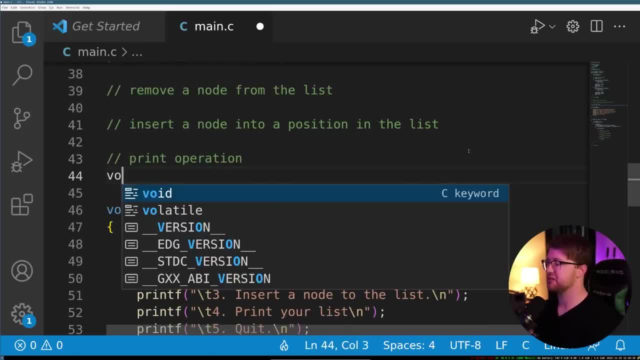 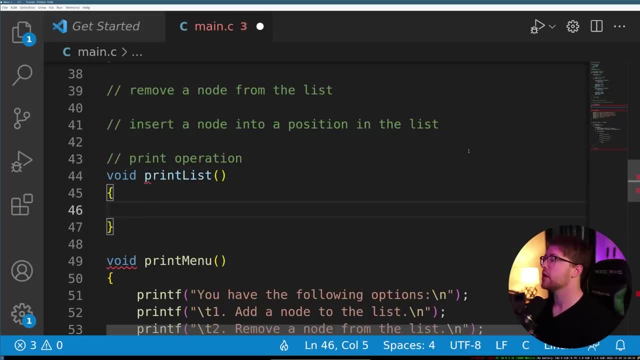 create our print operation first. so this is actually pretty simple. we'll make this a void because it shouldn't do any operations on the list. i don't need it to return anything to me. we'll say: void print list. and what print list will do is. it'll say: node pointer: current equals head. 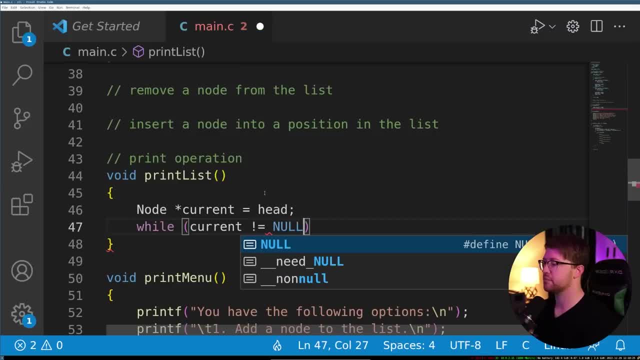 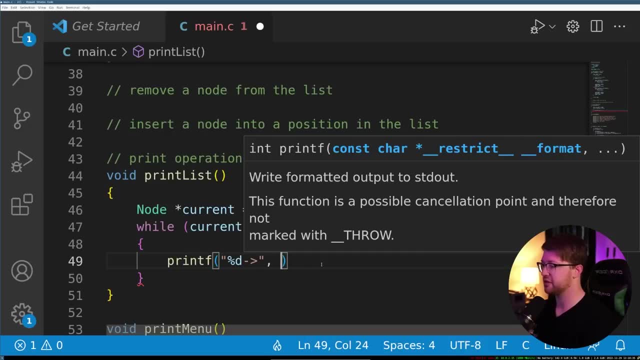 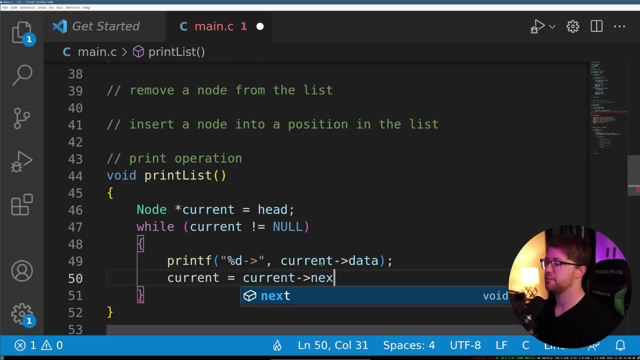 while current is not equal to null. print f, percent d and an arrow to make it pretty, and the percent d is going to be the current data and we'll say that current equals current next. so all we're doing here is we have a cursor that's walking across the list and after we do some operation on the current position in the list. 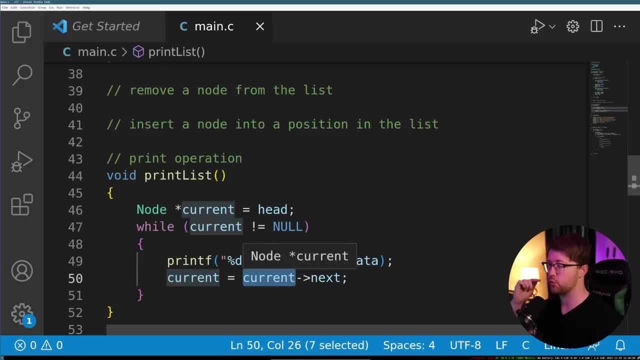 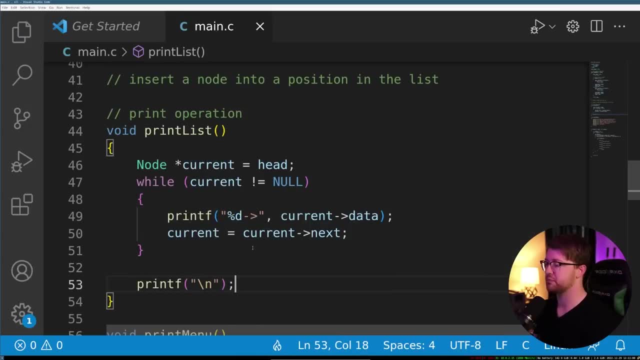 we make the current pointer equal to the current next point. we're walking forward one iteration on that list and then we say that we have to print f, a new line to make the display pretty, and we return. that's it walking through this. we are going to now add: 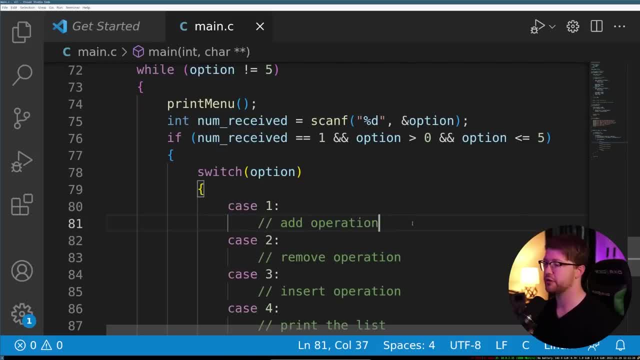 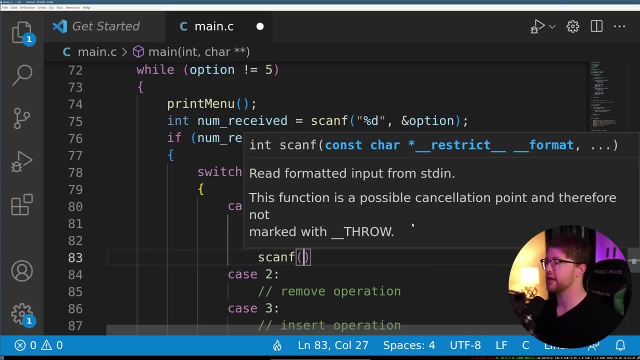 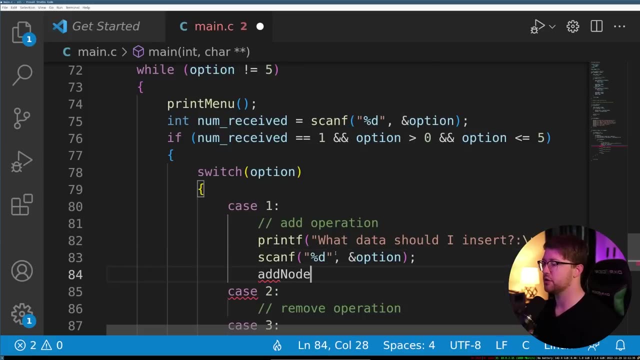 these operations here to our input and we'll go from there. so to do the add operation, we say to the user: what data should i insert? question mark, new line, and we'll scan f percent d again into the option field and we will say: add node, node new equals, add node and we're going to add 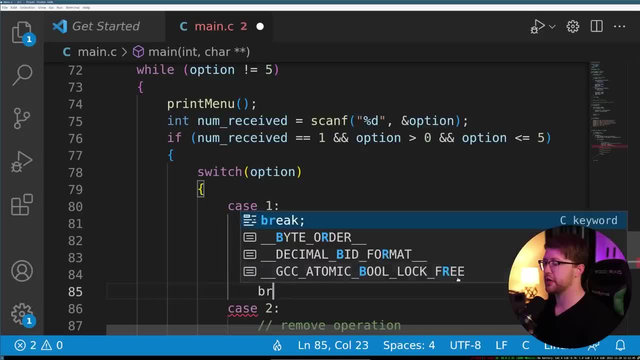 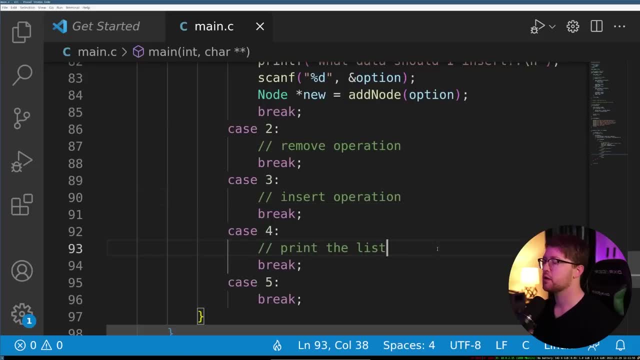 the option value. there we go. we have to break. don't forget to have a break statement, because if you don't, you'll fall through on your list. and then we're going to add some breaks here to make our code actually function. and then number four: if we get there, we're going to just reprint list operation. so 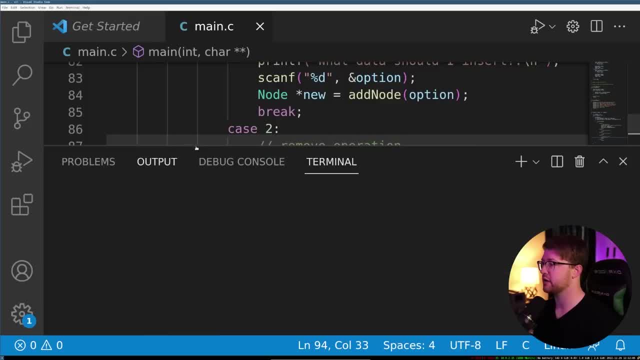 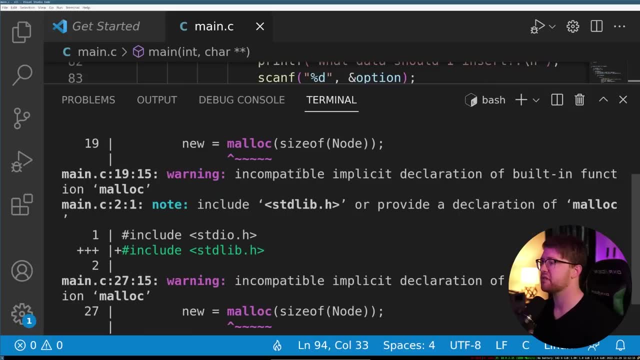 pretty straightforward, okay, so let's create a new terminal and see if we can't get our code to run. so gcc, tack o list on mainc. a couple errors here. these are all just warnings. i'm not including standard lib, so we're going to go ahead and include standard lib. 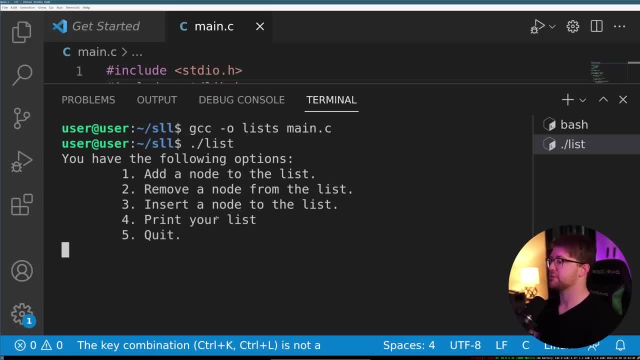 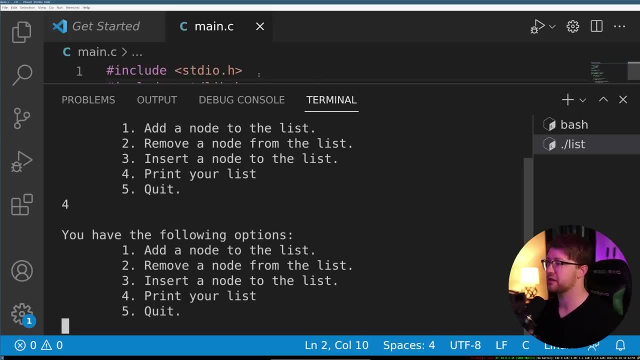 we'll go ahead and include standard lib, and we're going to go ahead and include standard lib. run lists the following options: we want to print the list, so this will actually crash. interesting though, because it says: while the current is not equal to null, and it's never. 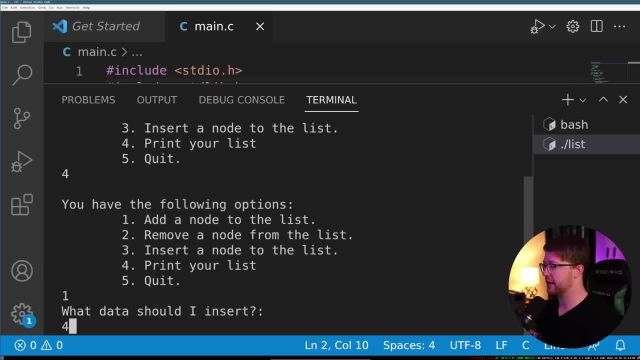 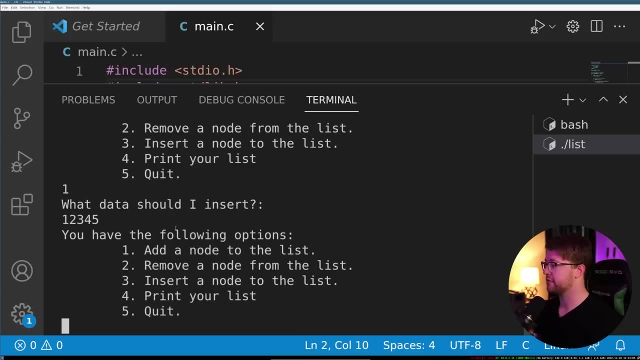 going to not be null, so it just immediately returns. okay, so add a node to the list. we want to add four to the list. we've added four. now print the list. we printed four. add a node to the list: one, two, three, four, five. now we print the list again and we have one, two, three, four, five and 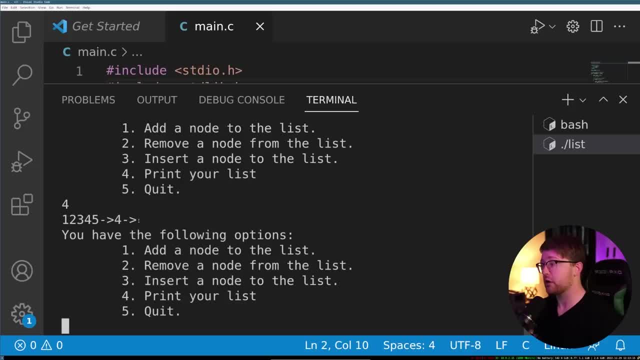 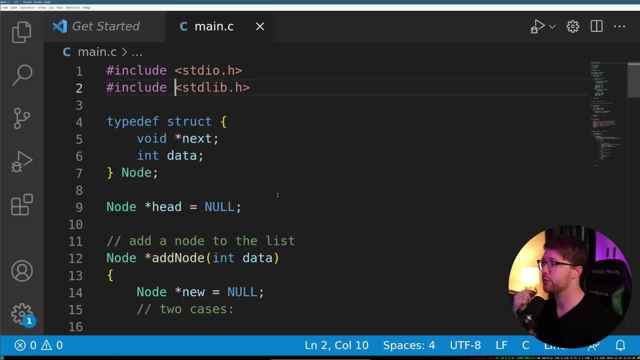 then four again, remember: it adds it to the back of the list. so, okay, cool. so we have done the thing. we made it a list and we made the ability to add a node to that list arbitrarily. that's great. next we want to do the next operations in our linked list. we want to be able to remove a node from the. 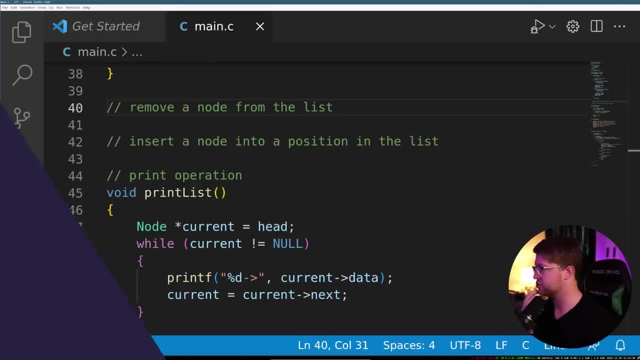 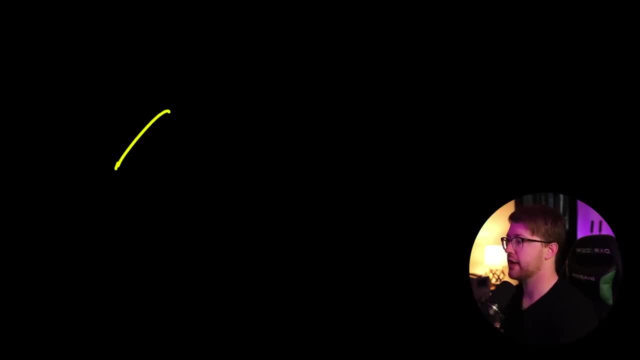 list. what is the removal operation on a list? let's draw it out. so let's pretend we have a linked list that has the following nodes: we have our head here. the head points out to element one and then element two and then element three. we are going to remove the list from the list. 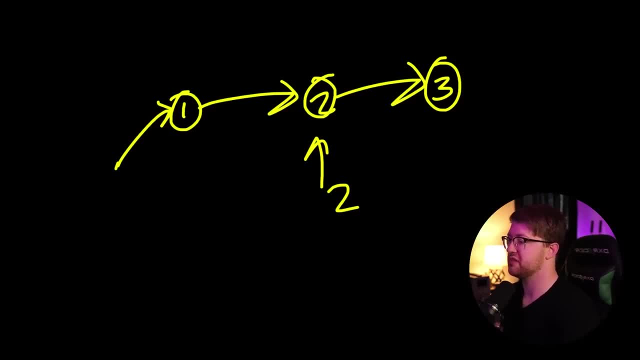 we are going to remove element number two from the list. so the way we have to do this is we have to actually walk it and track a previous pointer, because when we find element two, effectively all we have to do is make the previous pointer point forward to the next pointer. that will effectively. 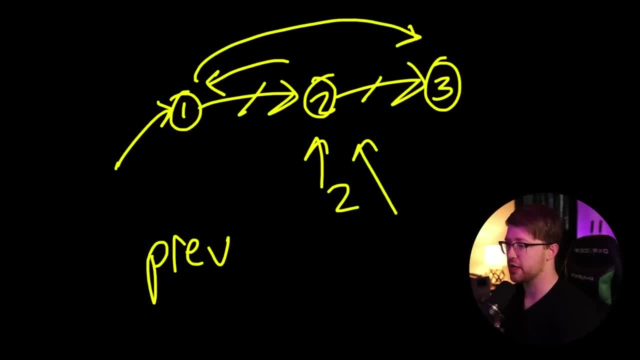 remove the links from the list and then we free this node. so we're going to do is we're going to walk the list and we're going to say: get to this element, track the previous, so the previous. at this point points to head: is this thing equal to two? no, okay, move on and we keep moving forward. 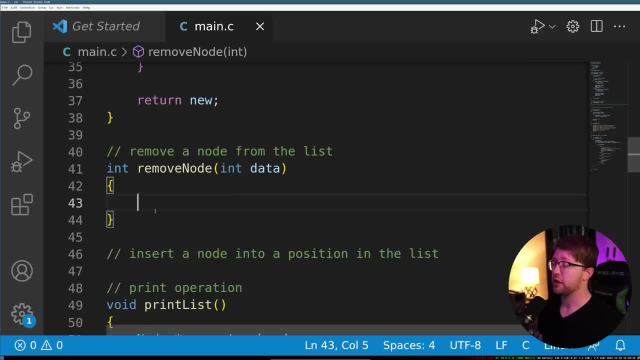 until we get to that point in the list. so let's do that right now. okay, so let's write the algorithm for removing a node from the list. we have to do the same kind of thing that we did before: we keep a current node on the list and we start with the head of our list. we're going to do is we're going. 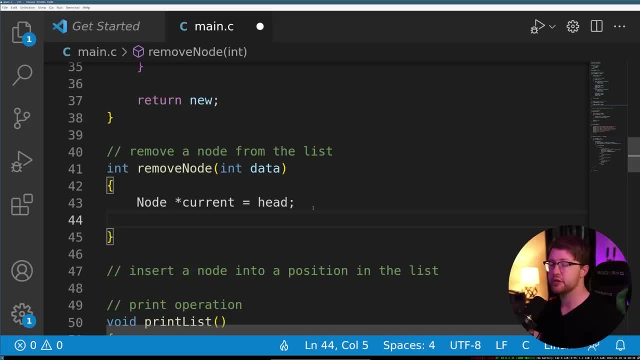 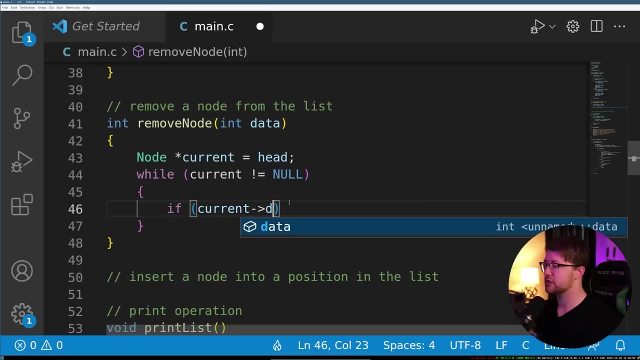 to walk through, starting at the head, and compare the data to our, to the data that we're looking for, and if we match, then you know we delete the node from the list. so we say, while we're looking for, we say if current data is equal to our data, the data from the user we have to handle. 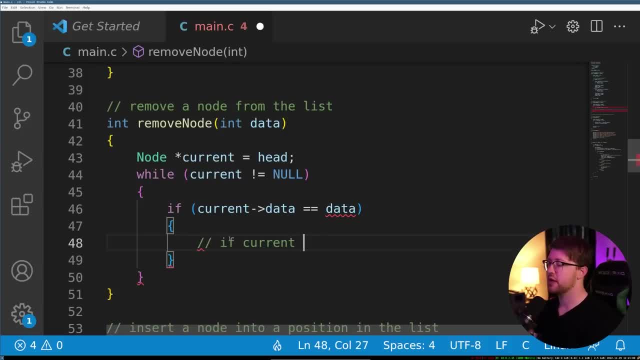 two edge cases. one is if the current node is the list head, because that changes the algorithm, we have to do right. if the current node is equal to the list head, then all we really need to do is just move the head of the list to the next element. so in this case we would just make the head equal. 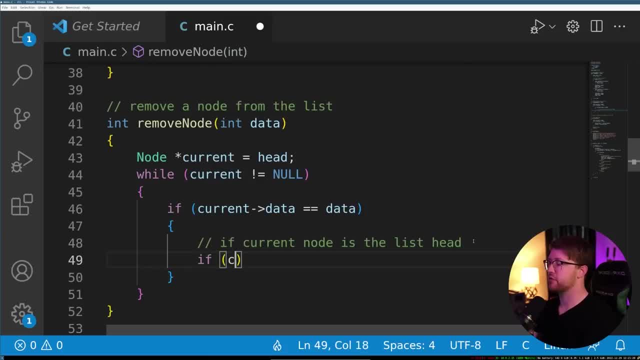 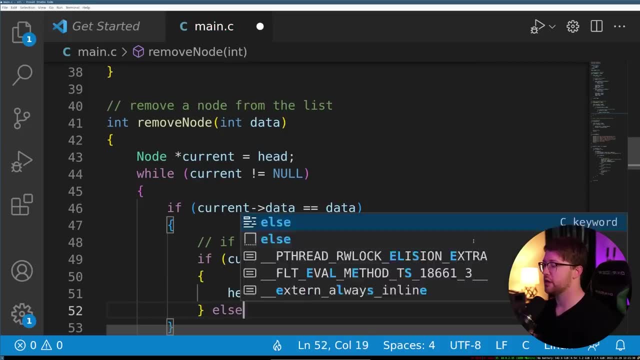 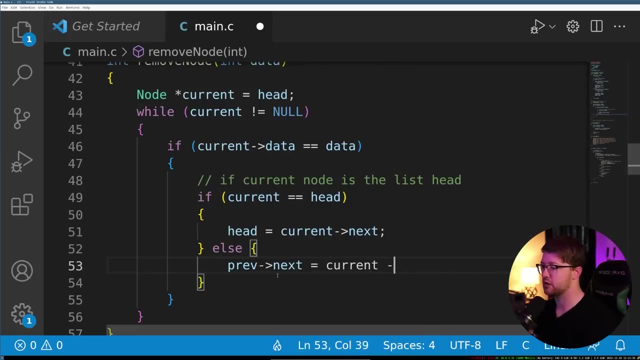 to two, which is our next pointer. so if current is equal to head, then we say that head equals current next, and then otherwise, if it's not, we say that we set the previous next pointer equal to our current next pointer. what we have to do is actually create this previous pointer and we can actually set it to start. 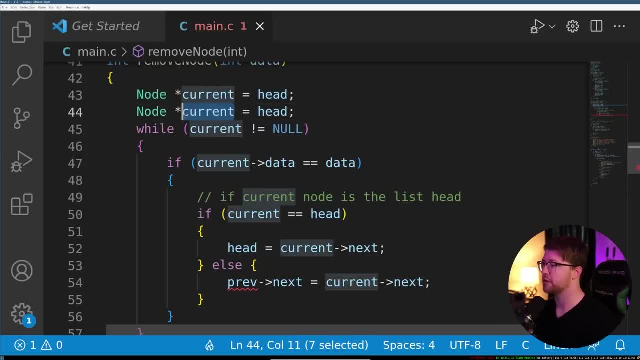 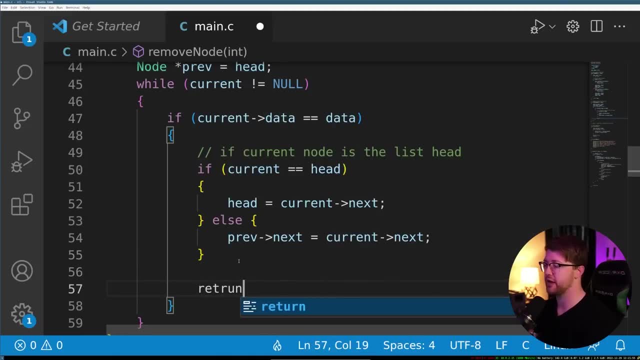 at the element head as well, and in either of these cases, if we found our data once we've removed it, we have to return back to the list head and we can actually set it to start at the one. tell the user: yep, we found the element in the list, so otherwise, if the data is not found, 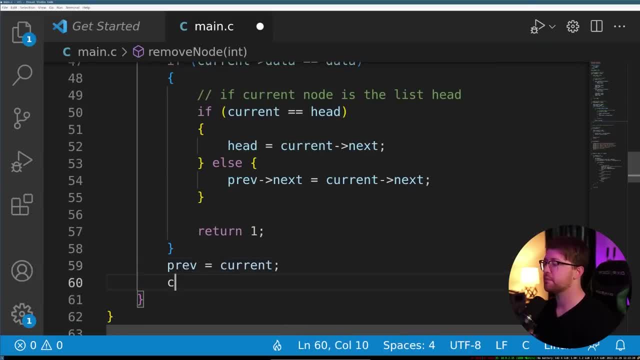 we say that previous is equal to the current node and the current node is equal to our next node. so we're tracking these two elements where one is always one step behind and the current node moves up one, and then eventually, if we get to the end of the list and we hit the front, the very end. 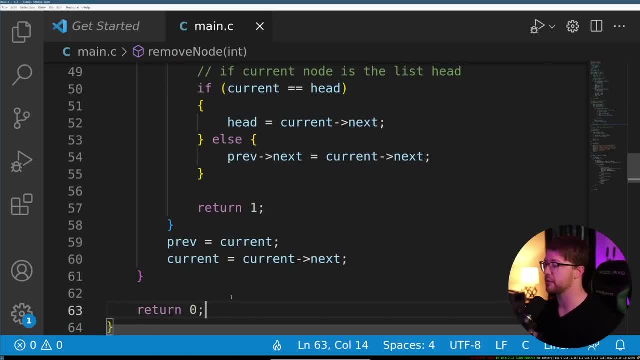 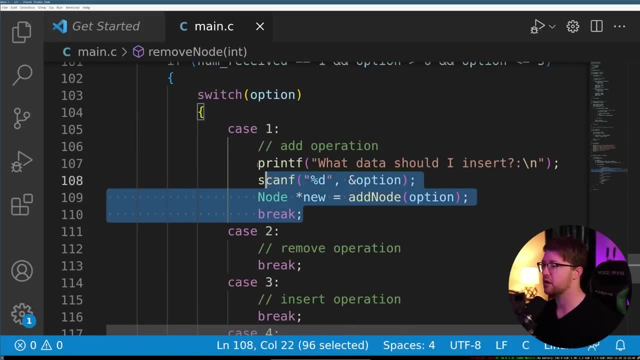 of the list where the list head is equal to null, we return zero, meaning we did not find it. so we're going to go ahead and implement this on our list and prove that it works. so we'll take all this code here and add it to the remove option. we'll 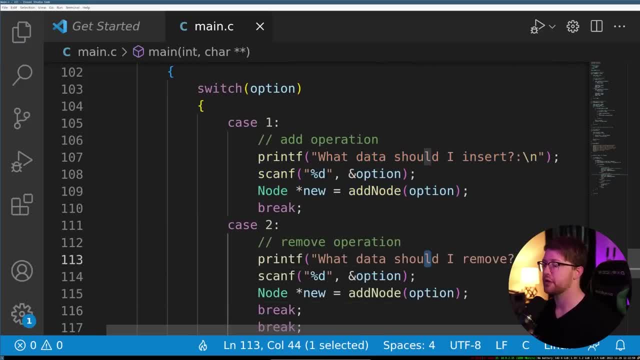 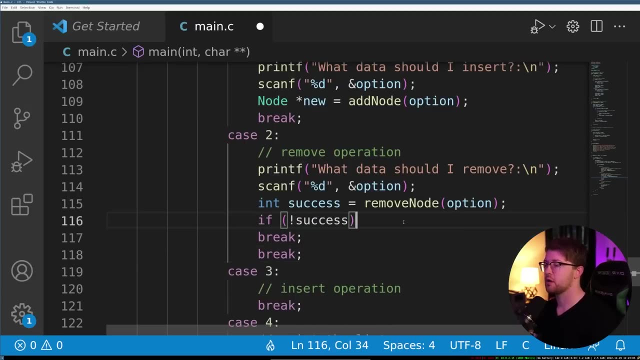 say: what data should i remove? i would like you to remove this node here, and it's not going to be a node pointer, it's going to be int success and we'll say: if not, or if not success, we'll just print out element not found. get rid of our second break. 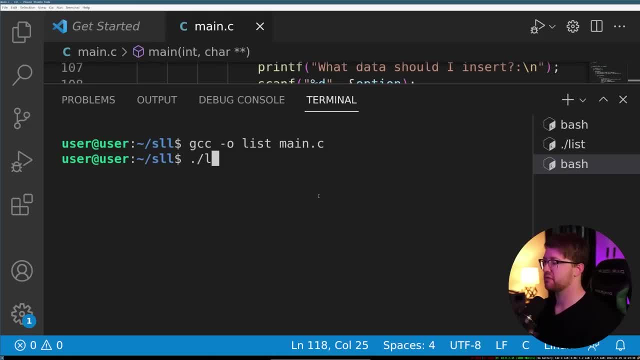 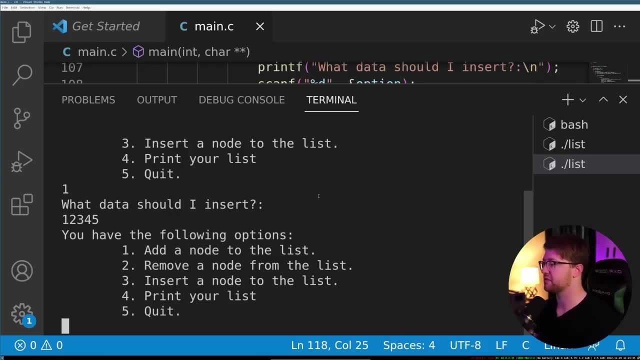 here and there we go, boom. so let's try this out. no errors, we're on the list. so we're going to add one, two, three, four five and we'll see if we can just remove one, two, three, four five from the list. one, two, three, four five, okay. so what if we print our list now? okay, so the list is empty, which is: 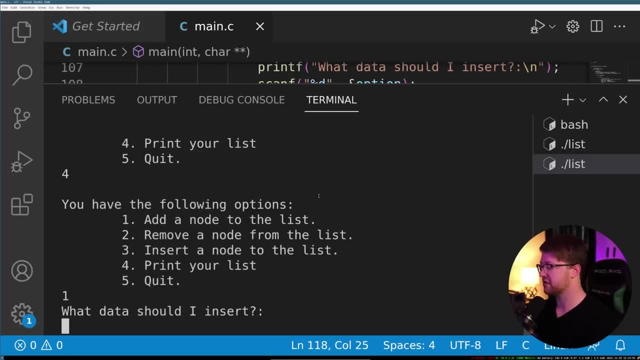 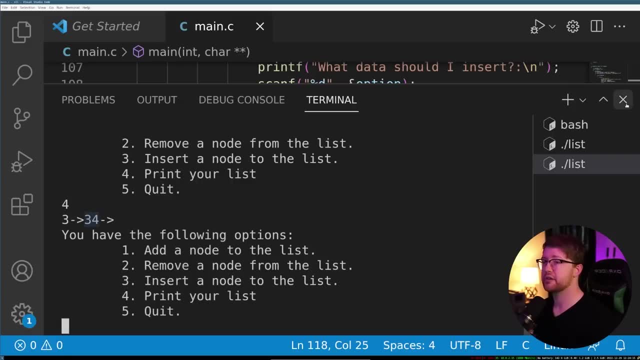 good, add a node to the list. one: what data should i insert? we should insert 34. let's print our list. okay, 34 works and cool. okay, so we removed it. the one issue that i just realized: we didn't actually free any of the data that we had in the list, so we're going to add a node to the list and we're 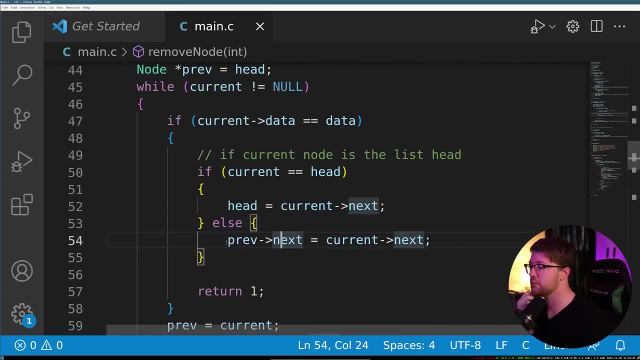 going to add a node to the list, so we have a memory leak on our program. let's actually fix that real quick. previous, next equals current, next. now we get to free current and set current equal to null, so that we don't ever have access to that again. there we go. we're done with the 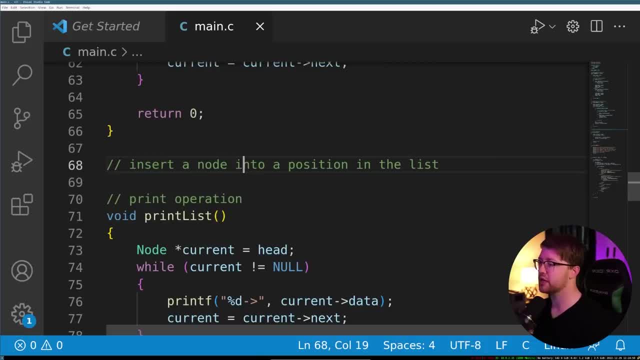 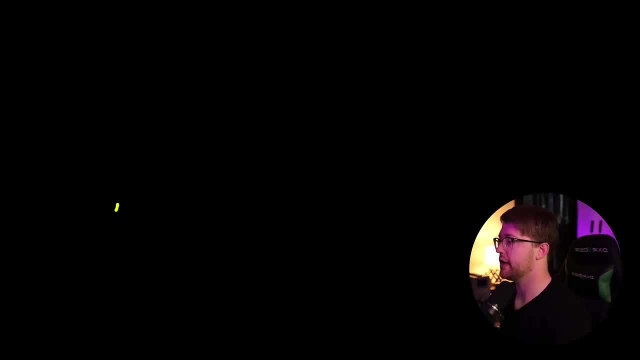 remove node. now we have the final operation: insert a node into a position in the list. so this one's pretty simple. we have our head. it points out to a position, of node one and this is position zero. let's say position two is position one, or data two is position one. 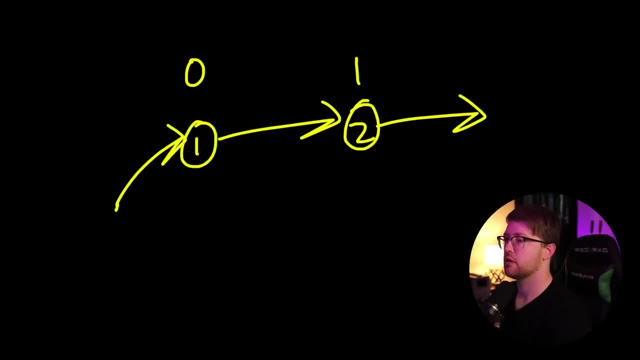 we want to insert in between these two, right? so what we can do is we create our new node, that is, node number four, and we're going to insert it into position one, which means we'll put it in front of node number two. so what we'll do is we'll just say that we make this new node. 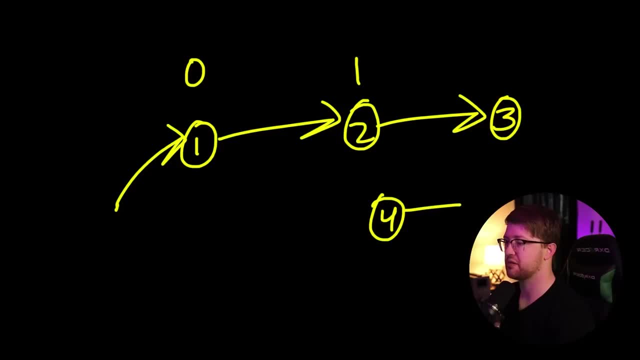 the new node is equal to the current next. so it'll point out to node three and we'll say that the current next is equal to us. so we're going to effectively remove this link, which is exactly what we want to do. so let's make that. 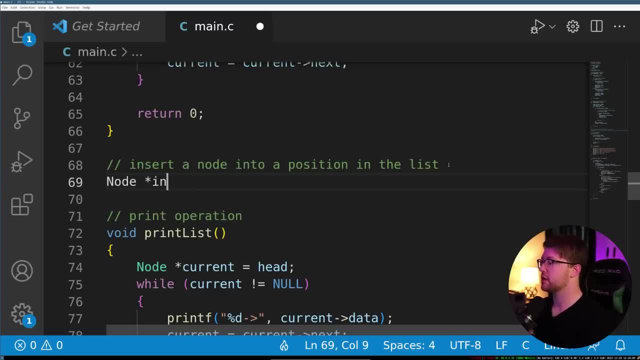 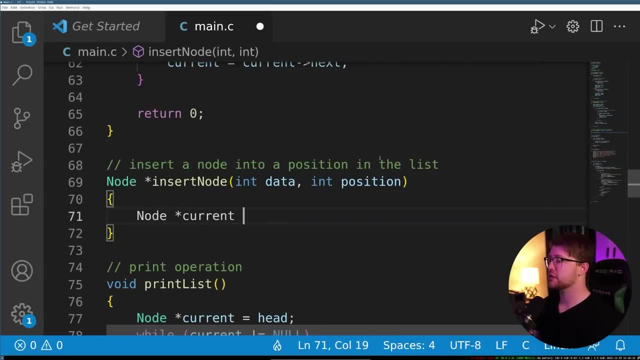 happen in c. so we'll say node pointer, insert node int data into position. we're going to say that node current is equal to head and we're to say that while current is not equal to null, position is not equal to zero. we'll just get position minus minus if we get to this position here and we say that if position 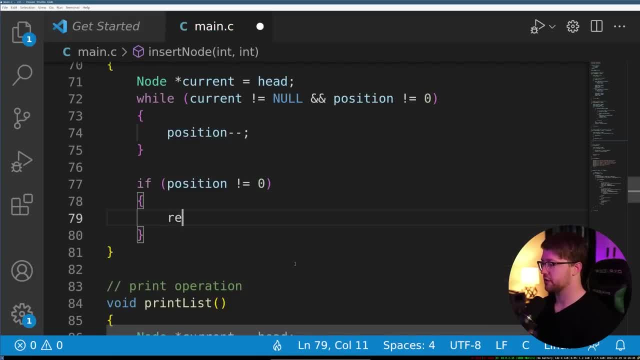 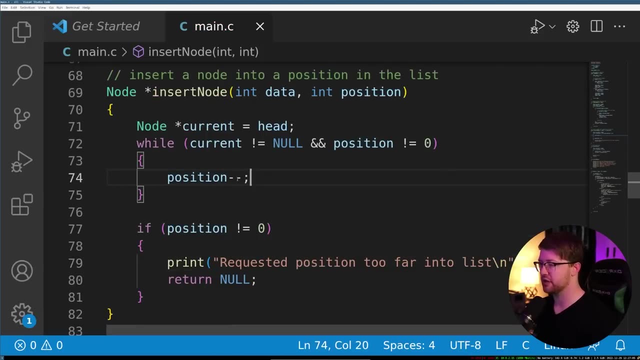 is not equal to null. to zero, we return null and we print out that requested position too far into list. because what happens here? if we get to this position here? in this loop we're iterating over the entire list until position becomes zero. if we get to this position here and we say that if position is not equal to zero, we'll return null, 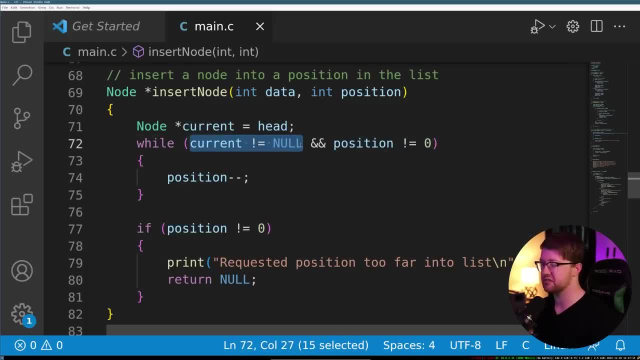 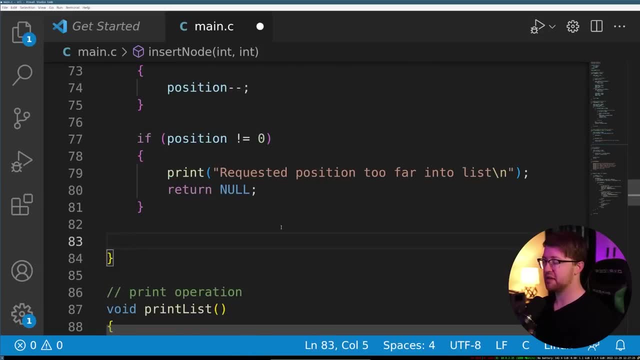 here, and it's not zero. that means we've encountered the end of the list before we meant to, which means that we asked to go too deep into the list, so we will return null here. now, if we get past this point, we've successfully actually gotten to a point where we can insert our node into the list. 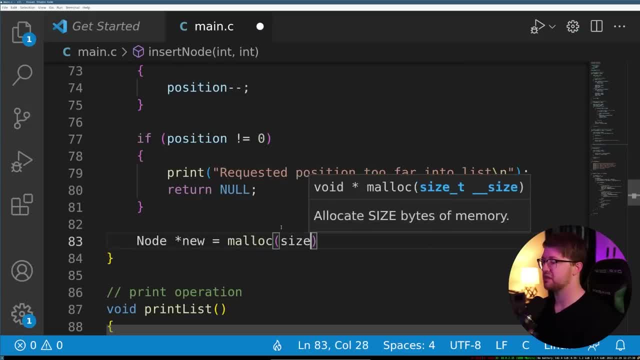 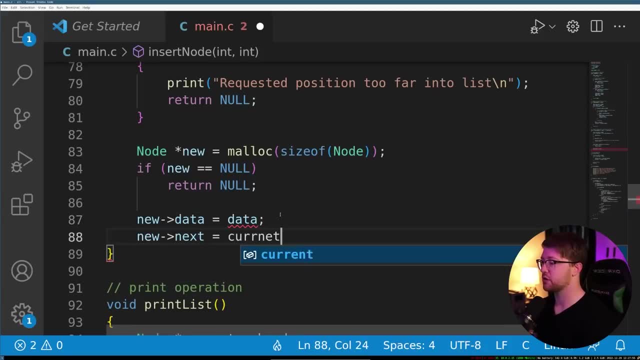 so we'll say that node new is equal to malloc. size of node new. node data is equal to data. say that the new node next equal to current next and we'll say that current next is equal to new. so that effectively points us to the node in front. 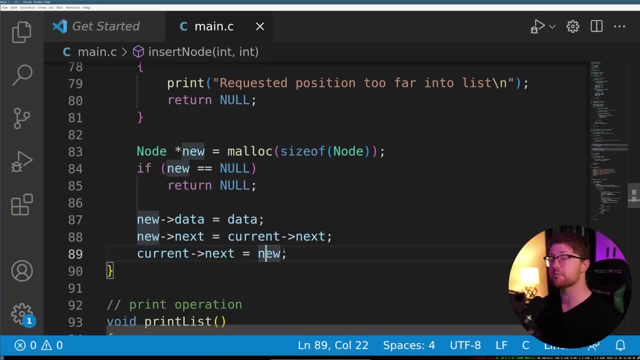 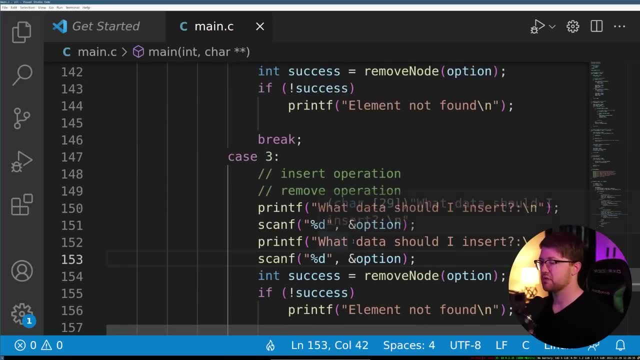 of our current and it points the current at us, putting us in the middle of those two nodes, and then we return the new node. so again, we'll do the same thing as before. we'll say what position, call it option two, and we'll say that node new is equal to. 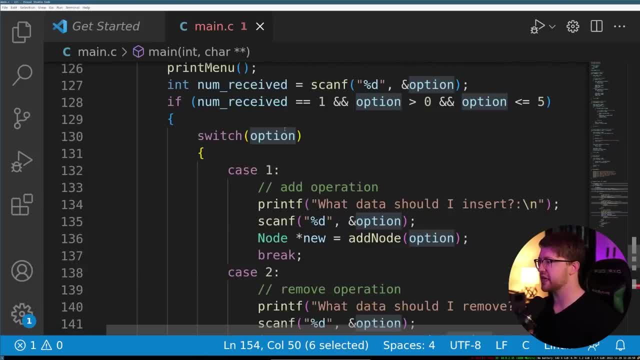 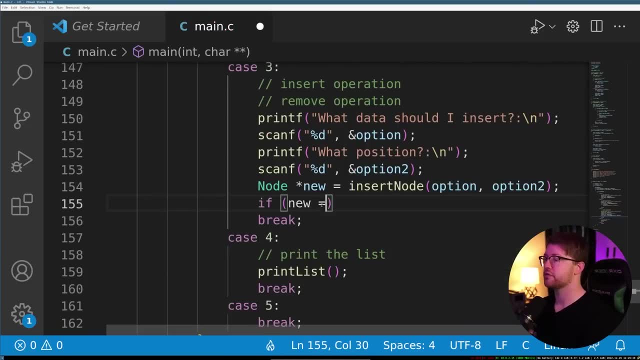 insert node and the arguments where i believe data and position right. data and position, yep. so let's say option. option two: we get null back. if new is equal to null, say, simply fail to insert into list, cool, all right, so let's go ahead and try that out. option two: oh okay, this should be zero and 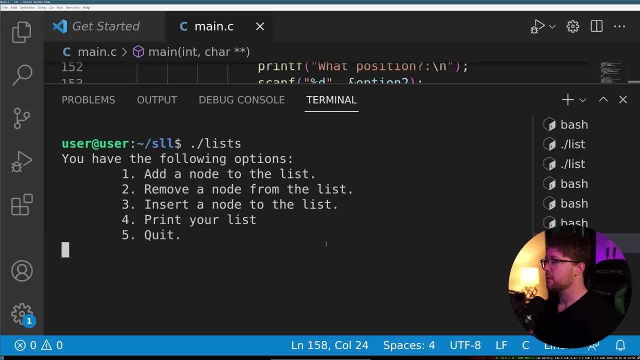 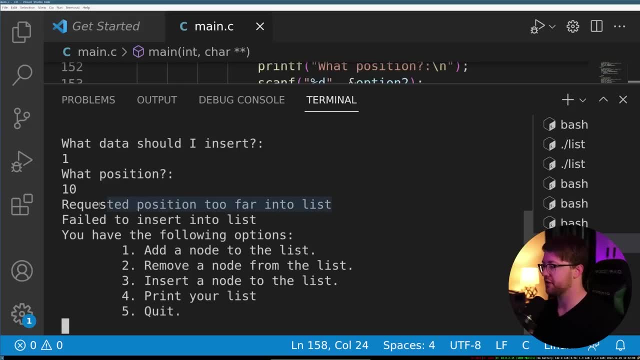 not null, but that's fine. so let's go ahead and run it. uh, first let's try to add a node to a blank list and then we'll say that node new is equal to data and position right data and position one, and then we'll say: insert data one into position 10.. so it's too far into the list. we. 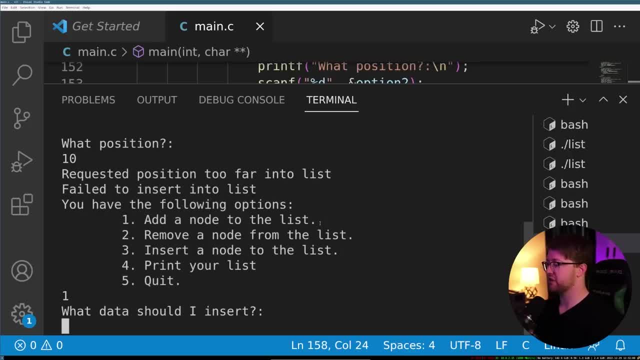 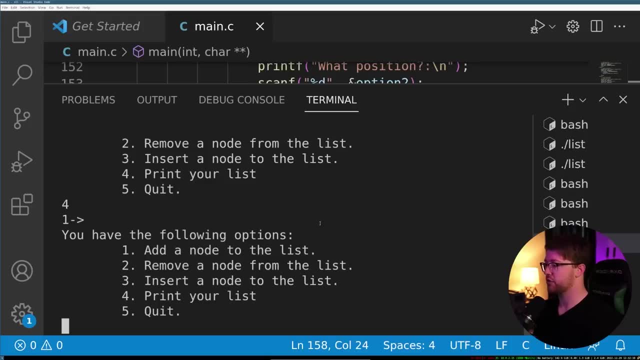 failed to insert into the list. okay, great, um, let's say: add a node to the list. we'll make the data at position one. we'll say the data will make it one, print our list. and we'll say: add a node to the list. i want to insert data four at position zero. i'll print our list out. okay, cool, so we put it at. 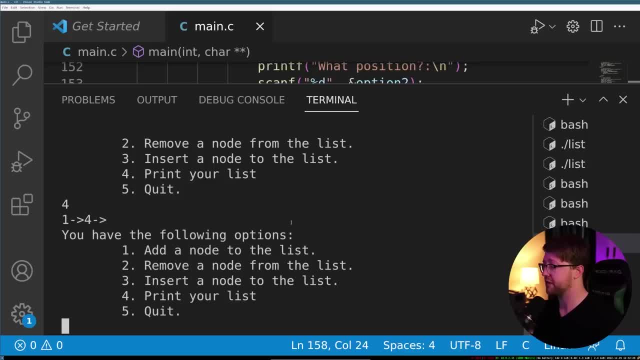 the end, or we put it at the front of the list. it's actually exactly what we want. that's awesome. um, now, let's say, remove data one, print the list four. now i want to insert data five at position zero. aha, so it crashed. okay, so we did. 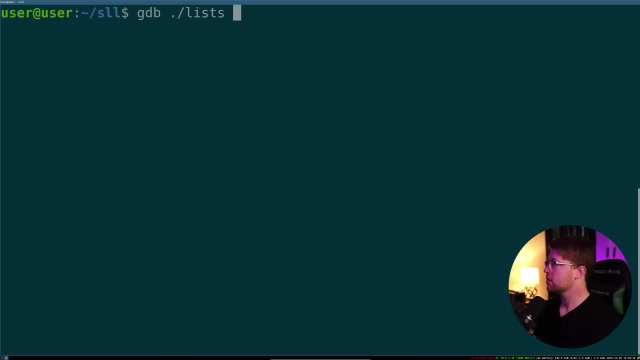 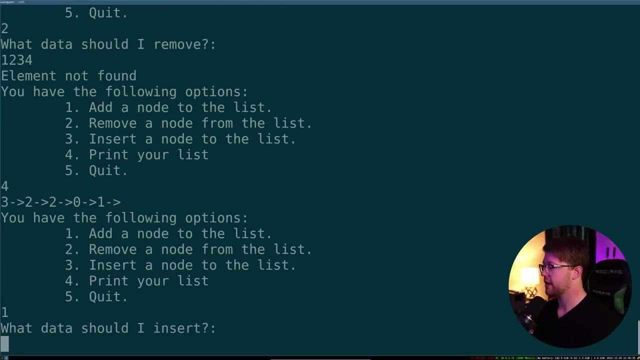 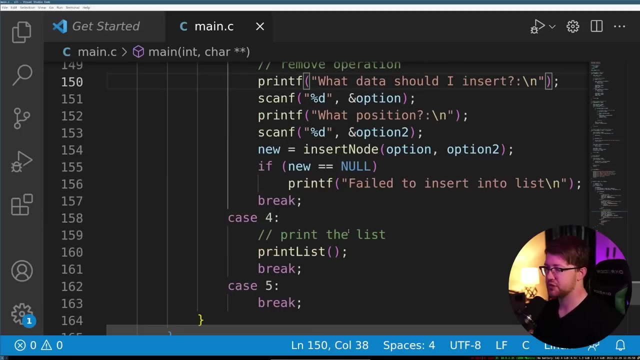 find a error. i believe we're gonna try it out in gdb and see if i can get that error to happen again. um, let's see, let's do add a node. oh, it's because i typed freaking five, dude. that's the issue. okay, so the issue is, if our option is five, if we ever use the number five in any of our 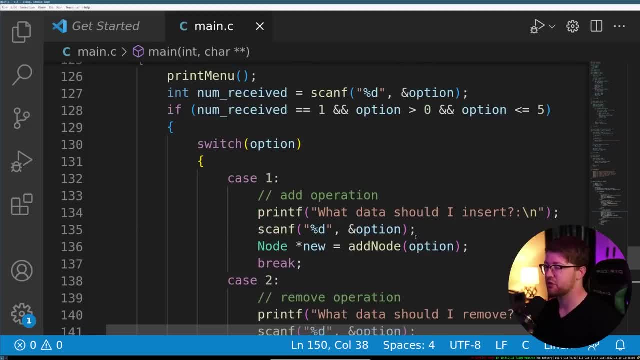 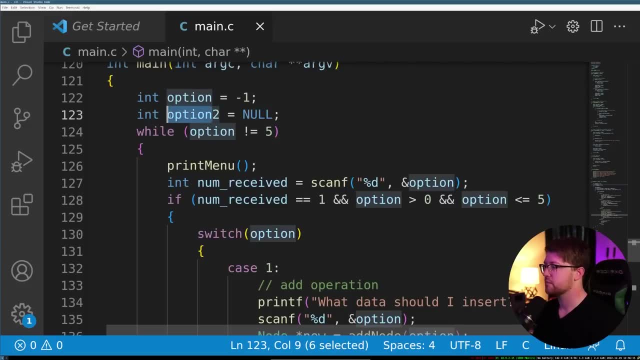 arguments it could be wrong. so let's say: add a node to the list. and we'll say: add a node to the list, it crashes the program. uh, that's interesting, it doesn't crash it, it properly does what it's supposed to do. hmm, yeah, we're just gonna make a new. call it arg1, arg2, zero, zero. because if we put